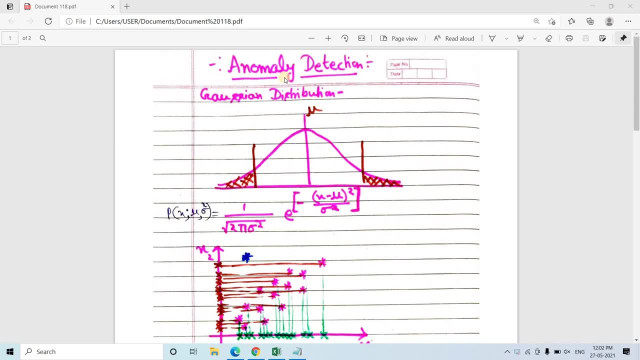 understand. Anomaly is nothing but outlier. okay, a rare or unusual observation in our data, Like for example in credit card transaction, fraudulent transaction, are anomalies because those are very few compared to normal transaction and those are quite different from normal transaction. 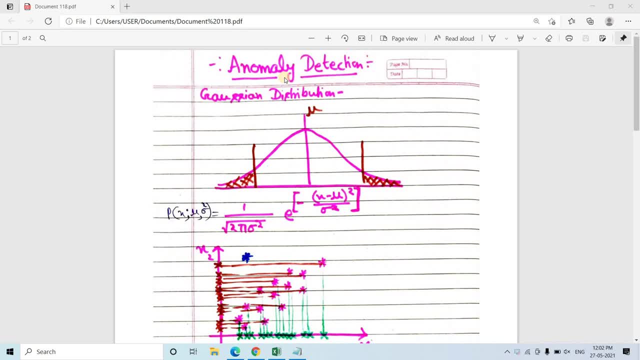 So those can be considered as outliers or anomalies. Now let us try to understand how we can detect those. Okay, so there are several techniques which I covered while discussing outlier detection techniques in the data pre-processing stage of data science or machine learning projects. right, One of the popular technique which I covered is three sigma rule. 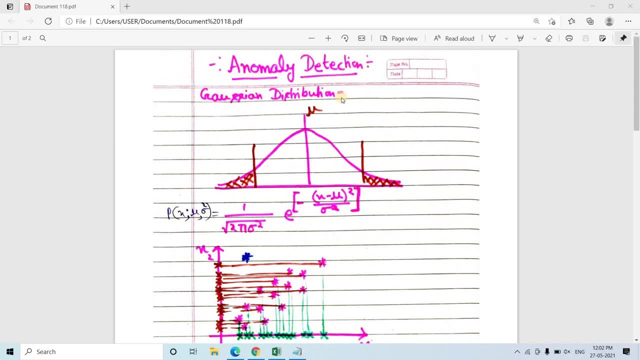 that is, basically compute the z-score for our that data point, and if the absolute value of the z-score is exceeding three sigma, that time we can consider that that particular data point is an outlier. Okay, so the picture can be shown like this: Suppose I am having some data points I try to fit. 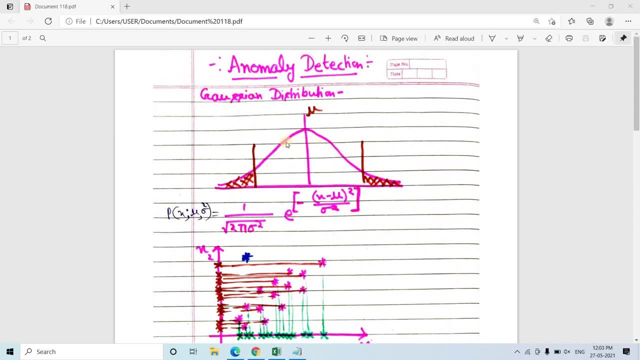 a Gaussian distribution data. I try to compute Gaussian distribution for those data points. okay, which is having mean as mu and standard deviation as sigma. So the probability distribution or probability density function looks like this: 1 by root over of 2 pi sigma square multiplied by e to 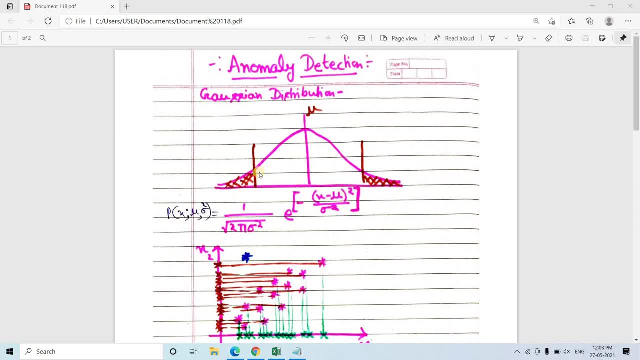 the power minus of x, minus nu, whole square by sigma square. right Now, what I have told you: minus 3 sigma to 3 sigma. if some data point is, if the z-score of the data is falling under that region, that can be considered as normal data point. But if the absolute value of the z-score 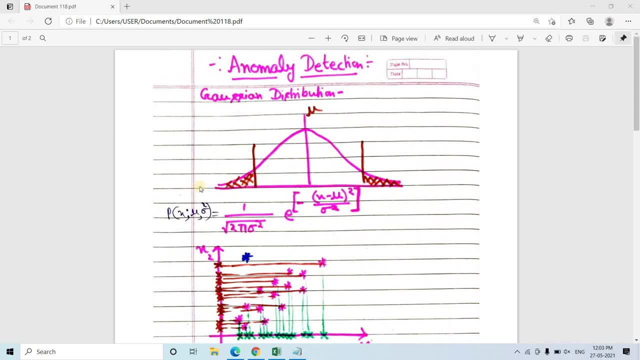 is exceeding 3 sigma, that is in negative side, it is going beyond minus 3 sigma in the left side direction, or in the positive side, it is going beyond plus three sigma in the right side, then this particular, those data points will come in these shaded regions and those can be considered. 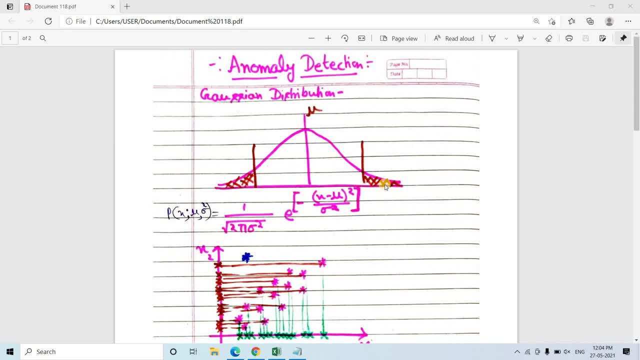 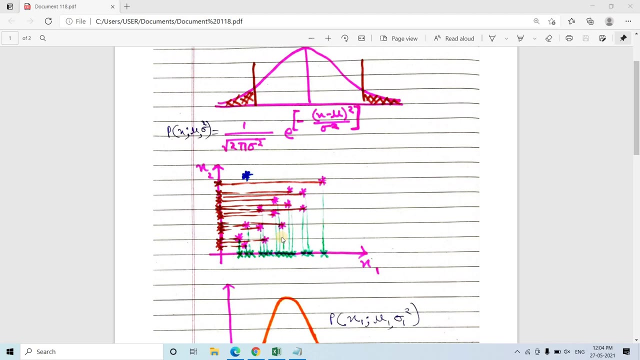 as outliers. right Now let us try to map the same concept in higher dimension. So in this video I am going to discuss in two dimension, outlier detection or anomaly detection. okay, So you can consider the data, the scatter plot of our input data like this: okay, So there are two input. 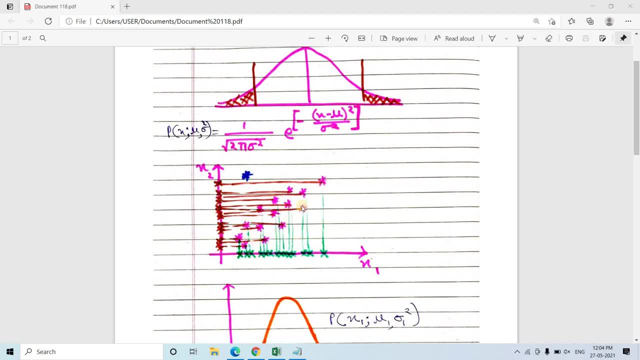 features x1 and x2 and if we draw this scatter plot, we will be getting this data. okay, and this blue colored star is also included in our data set. So from the visual inspection itself, we can clearly conclude that this blue colored data is basically going to be outlier, because this- this: 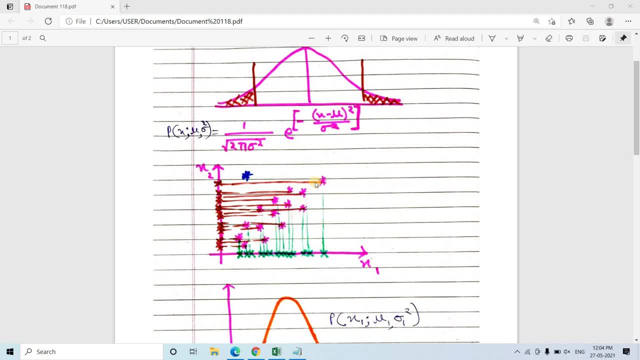 is quite different from the data set. So we can clearly conclude that this blue colored data is from rest of the data points, Rest of the data points. in between x1 and x2 feature there is a high correlation. If x1 feature increases, x2 feature is also increasing. but this data point. 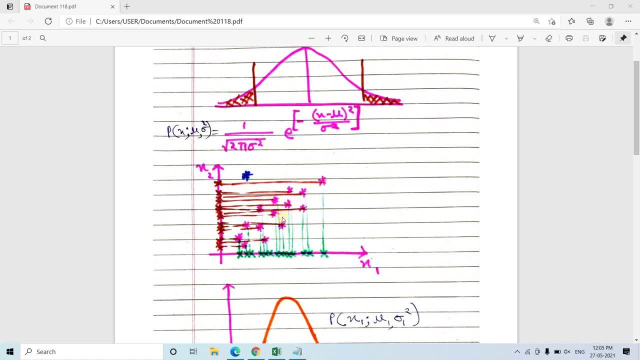 is not following that behavior and it is significantly different from rest of the data points. So we can easily say that this is an outlier. but how can we detect this? Let us try to understand So what we will do, like here in one dimension case, we computed probability, okay. 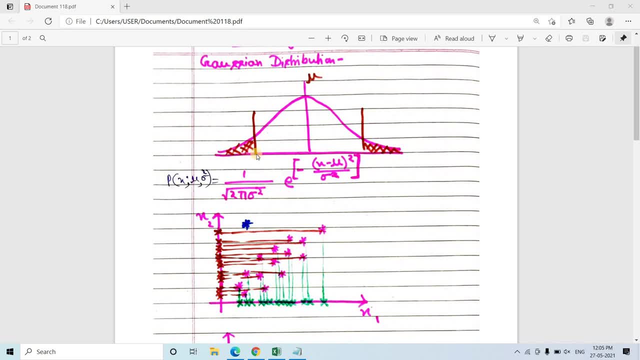 So basically, we said like this: it's just a probability, So we can easily say that this is a outlier. So we can easily say that if the absolute value of the z-score is exceeding 3 sigma, that time that can be considered as outlier. So what that means. okay, let us try to understand. 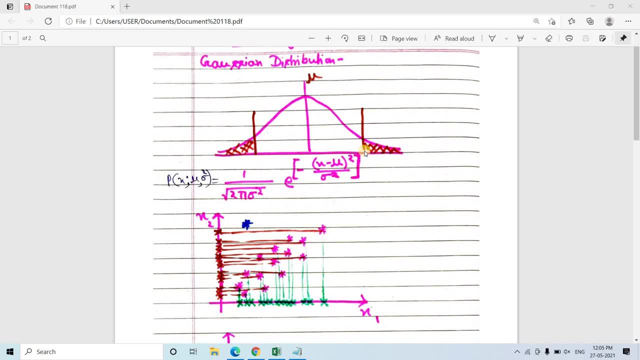 So here minus 3 sigma and here plus 3 sigma is present. suppose If we are going beyond minus 3 sigma or plus 3 sigma- that is this part- we can see that the probability of those regions is actually very less Higher. probability is concentrated within minus 3 sigma to 3 sigma. That's why it's. 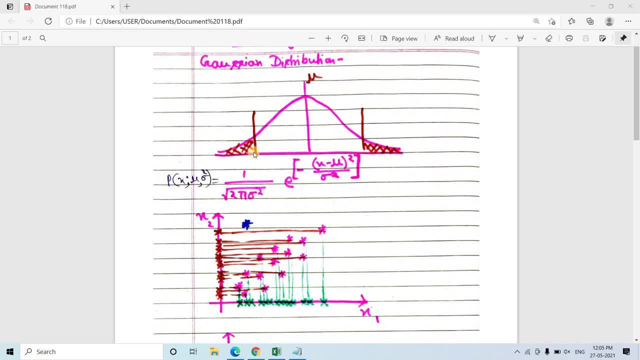 telling that if the data point is exceeding minus 3 sigma in the left side or plus 3 sigma in the right side, that in the probability from the Gaussian distribution itself we are getting very less. So that indicates that the probability of happening those kind of event will be less. 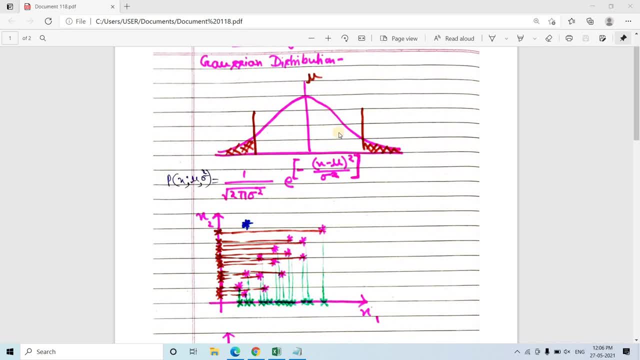 So we can consider those as outlier in one dimension case. Now, same concept we will apply in two dimension, but this is, there are two features. So we need to get the probability values for each data point, for with respect to x1 variable and x2 variable, and then we will. 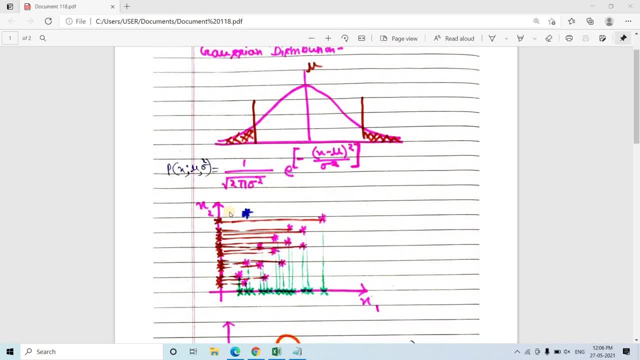 compute the overall probability, So how we are going to compute that? So for any data point, what is the probability with respect to Gaussian distribution? if you want to consider here, suppose, this data point. So we need to compute p of x1 comma, x2, considering x1 and x2 as random variable. 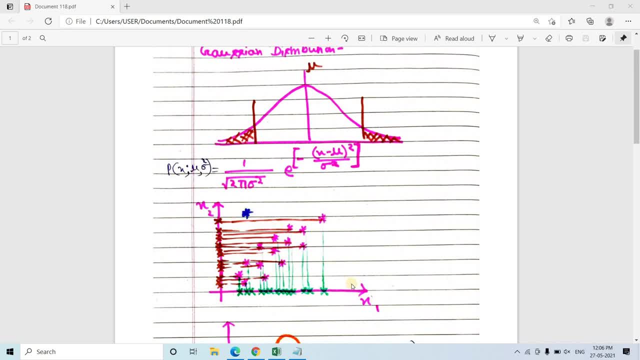 Now, x1 and x2 are what? x1 and x2 are our input features. Those are independent, right? Those should not be dependent on each other, right? That's what the fundamentals of machine learning says. So, probability of x1 comma x2, we can easily say: 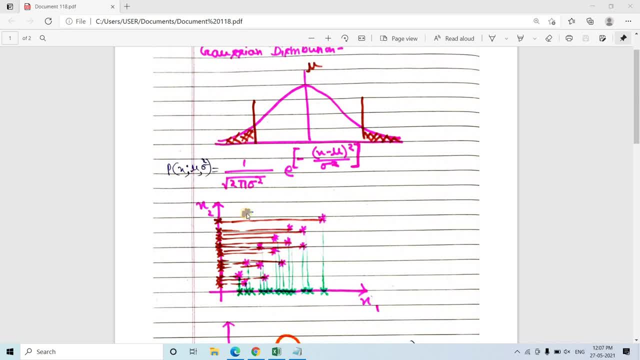 equal to probability of x1 multiplied by probability of x2.. So to compute the probability we can use this particular simple formula of probability and statistics, that is, probability of x1 comma x2, equal to probability of x1 multiplied by probability of x2 if x1 and x2 are independent. 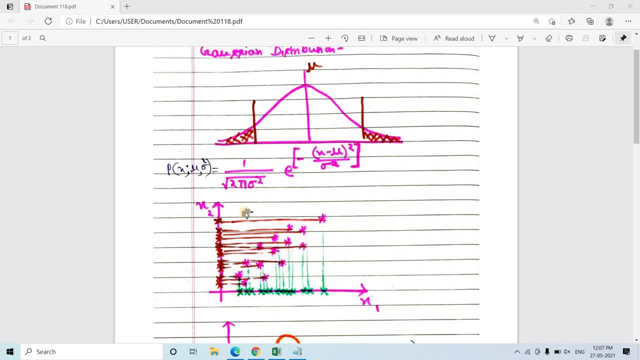 So what we can do to get the overall probability in these two dimensions. We will compute probability for any data point in the x1 direction and in the x2 direction we will multiply those, We will get the overall probability. and if the overall probability comes very less, how to. 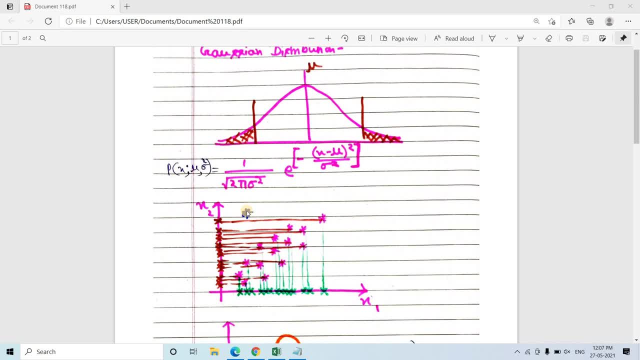 understand whether very less or not. so less, we can adjust one particular threshold and the threshold has to be chosen very wisely and based on that threshold. if the probability, overall probability- goes below that threshold, then we can get the overall probability. So, based on that particular threshold, we can consider that. okay, that is nothing but outlier. 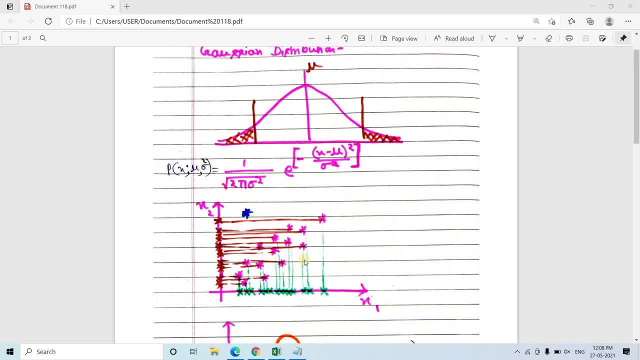 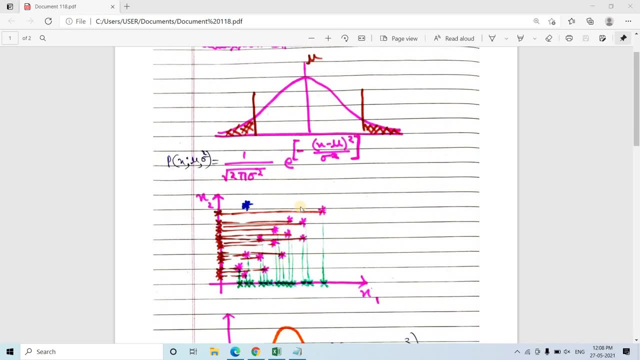 okay, like that we will go. So for any data point we need to compute first the probability in x1 and x2 direction. okay, How can we do that? Simple, these are our data points. take projection on x1 direction that these are basically x1 values for all these data points. 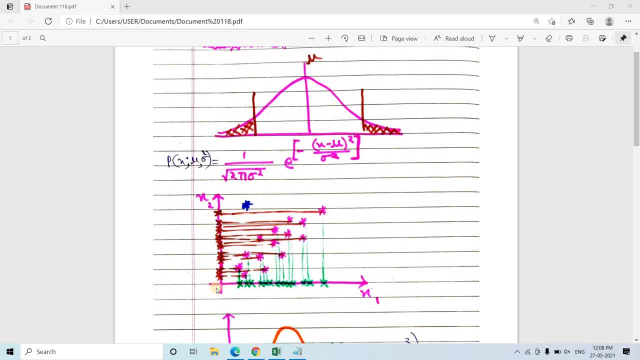 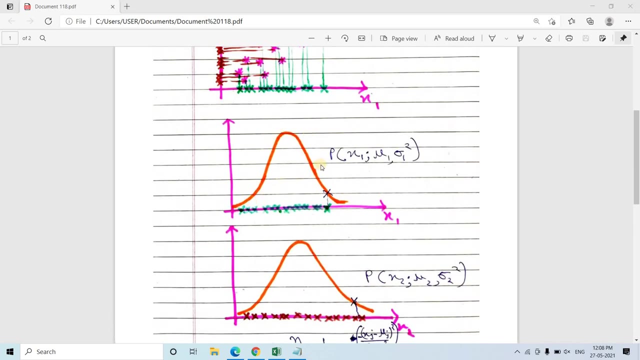 Similarly, take projection on x2 or y-axis. you will be getting the x2 values. Considering this x1, you make one probability Gaussian priority distribution. Considering this x2, you make another Gaussian priority distribution and the shape will look like this: So this Gaussian distribution is probability of x1. okay, All these projection along x1 direction. 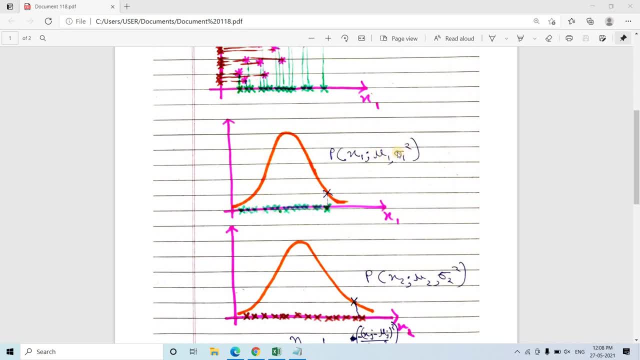 we have taken. we try to compute mu1, that is mean and variance, okay. or if we say sigma 1, that is basically standard deviation, okay. So once we get the mean and standard deviation for any data point, we can easily compute what is the probability right. Similarly, 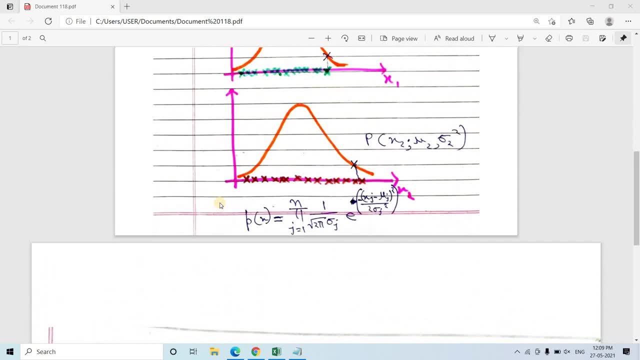 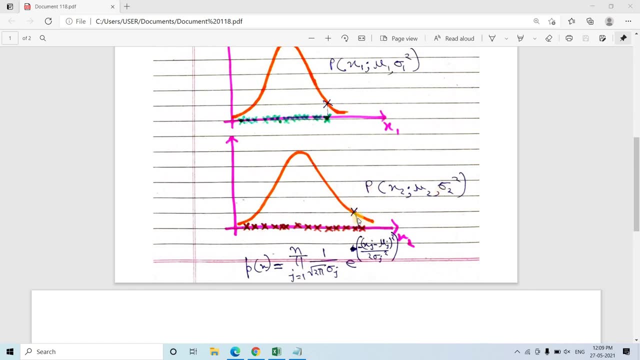 these x2 projection values we can take here, and then again we can compute mean and standard deviation and we can get what is the probability for any data point. okay, Like for example: suppose for a particular data point along x1, the value is this one, what is the probability? 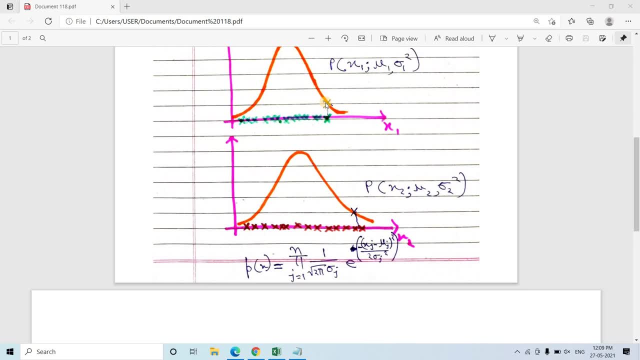 that is, this is the probability right. We can easily compute using that formula of probability. Similarly, like for x2 feature, any value is taking, like at this location. then what is the probability with respect to Gaussian distribution? that is this value right. So to get the overall 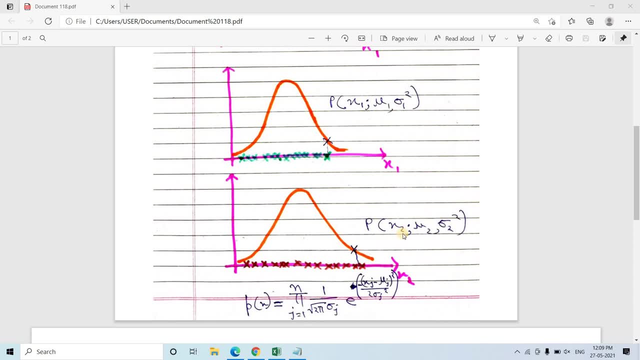 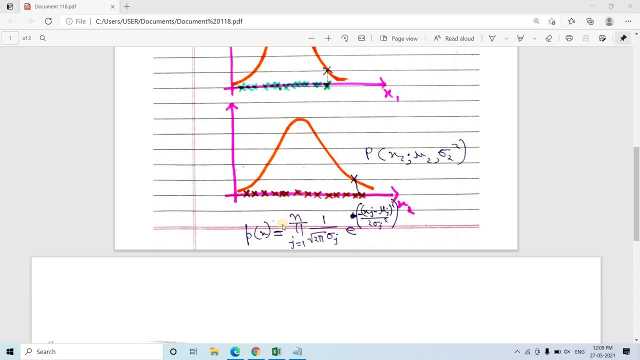 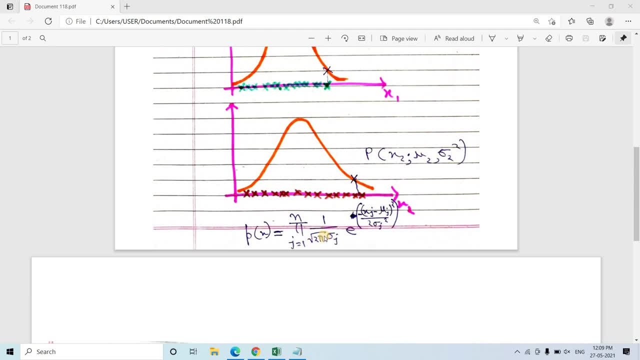 to 1 to n. y symbol. that indicates multiplication 1 by root over of 2. pi. sigma j: If you want to put sigma j inside root over, it will be sigma j square, as I have taken this sigma j outside the root over, so I kept like this. okay, Whatever mathematical notation you want, 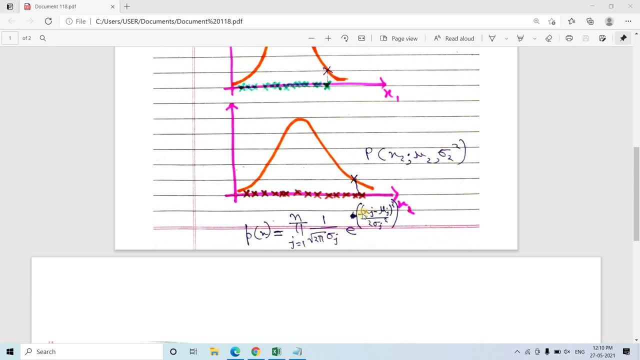 to use. you can use that. No issue in that, Multiplied by e, to the power minus of xj, minus mu j square by 2 sigma j square, What is this? j? J variable is basically indicating you that. So that means it's 100% positive or negative. but we just need to compute this. 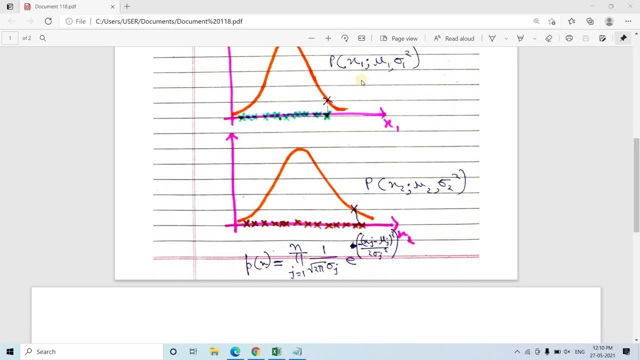 input feature. like there are two input feature in this case, so we are multiplying two probabilities only to get overall probability of each data point right. so n is total number of input features. okay, present in our data set which we are going to use for training our machine learning model. okay, 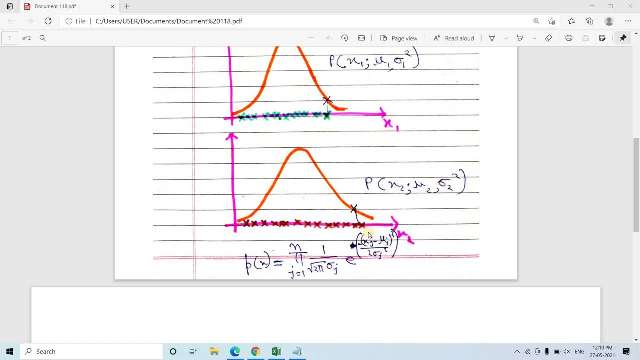 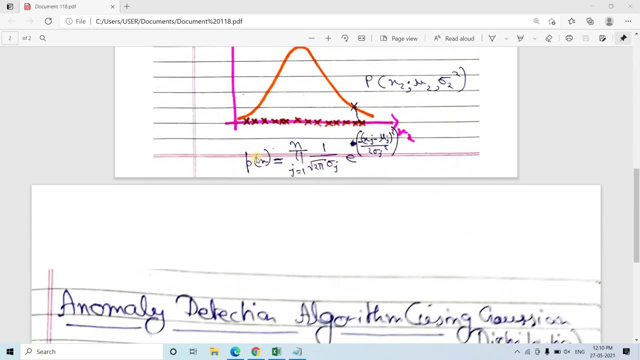 so like this: we can get the overall probability with respect to both input feature for each data point and then we can adjust a particular threshold. if the probability values- overall probability values- goes below that particular threshold, we can consider: okay, it is out there, okay, right or anomaly? so what is? 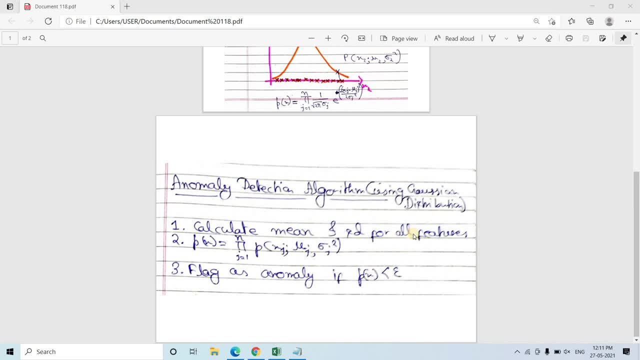 the anomaly detection algorithm using Gaussian distribution says: calculate mean and standard deviation for all the input features. okay, and then you have to. for each data point, you have to compute the probability. okay, P of X equal to J, equal to 1 to n. that is, for each input feature, what is the probability value? so we need to. 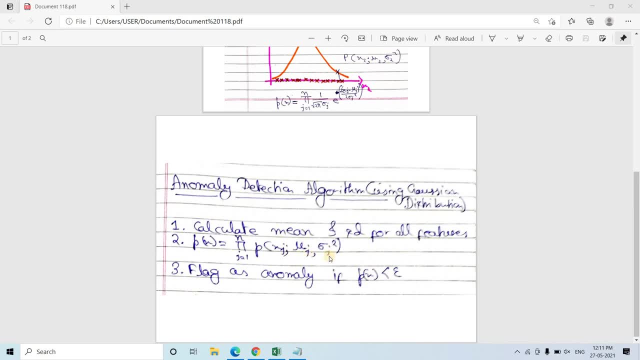 multiply okay, P of X, J and where a, mu, j and sigma j square are mean and variance respectively. for that particular jth input, feature okay And flag as anomaly with probability that is, overall probability less than epsilon. What is epsilon? Epsilon is a particular threshold which we will be using as benchmark for detecting. 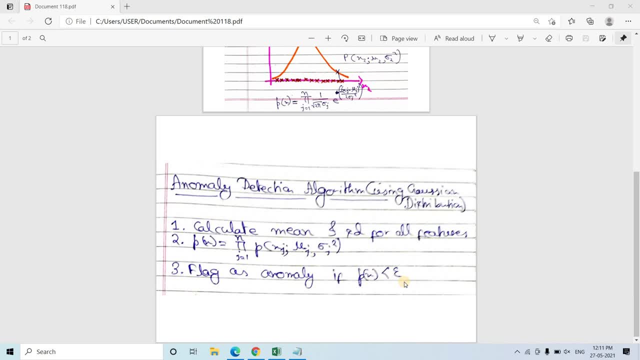 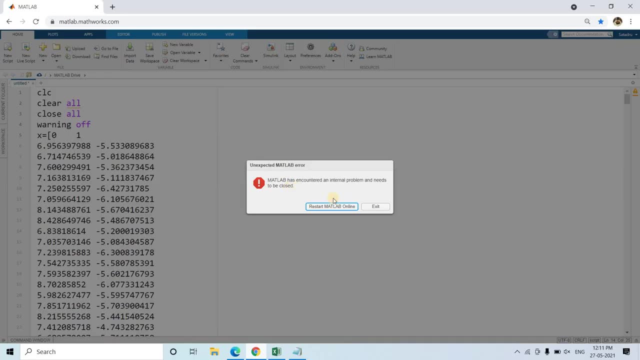 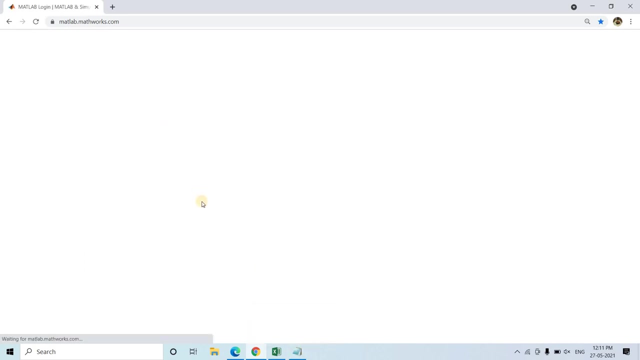 outliers. That's it. okay Now this theoretical concept. I hope you have got a feeling, but the feeling will be more clear once we go to programming. Let me show you that. okay, So here let me restart MATLAB online. I am using, So I have already written the code, Let me take. 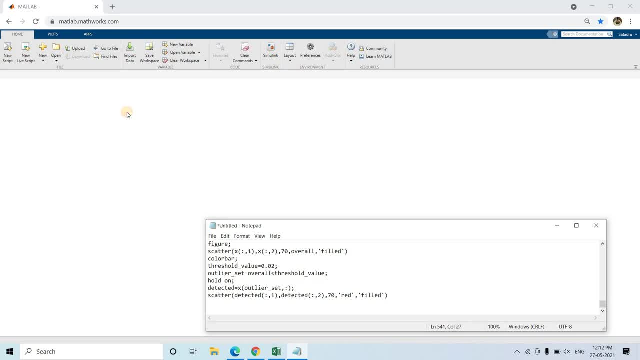 this particular code. once The code I will be providing in the description box or in the comment section, No need to worry about a single line of code. okay, Let us try to fill the idea with visualization first, because once we see the see what is happening mathematically. 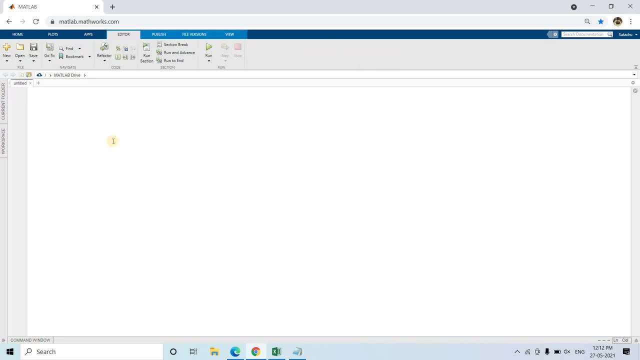 we are going to be able to see that. we are going to be able to see that we are going to potentially and programmatically, Then it is hard to forget the concept. okay, And concept is power, not the inbuilt functions or packages, Input pieces. this will not make a strong feeling, okay. 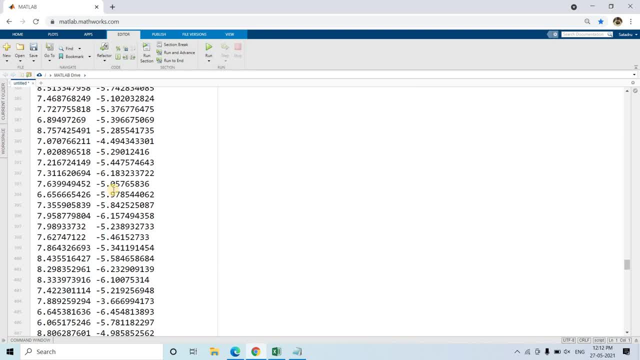 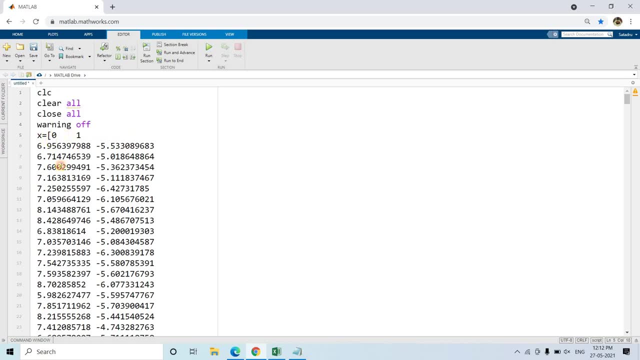 You can remember this visualization of the concept easily, Mathematical concept, whatever just now I have discussed. So what is the code? CLC, clear or causal, warning of simple. Now I have taken one two-dimensional data, X first input feature you can consider as x1.. 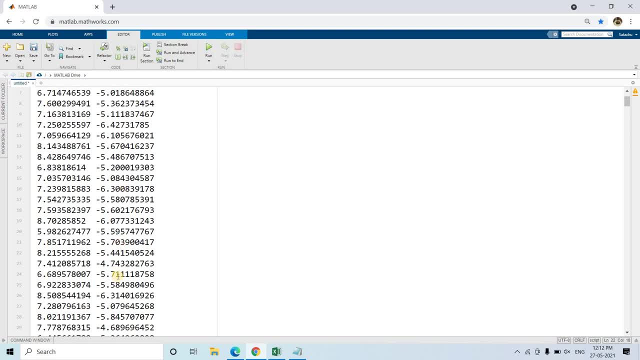 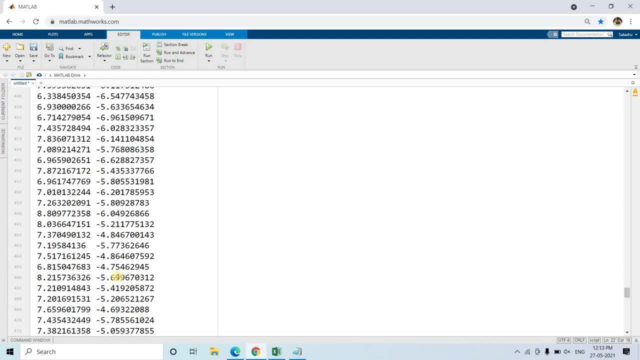 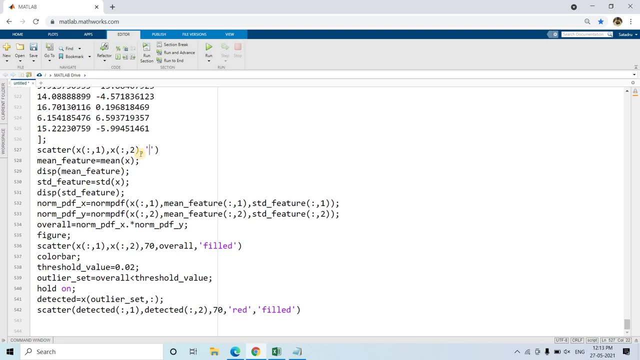 And second input feature. you can consider as x2, second column. Now here this is our data code will be posted, no issue. So you can try with that and the data is quite big. Now what I am doing first. I am first doing scatter plot. here let me give field. 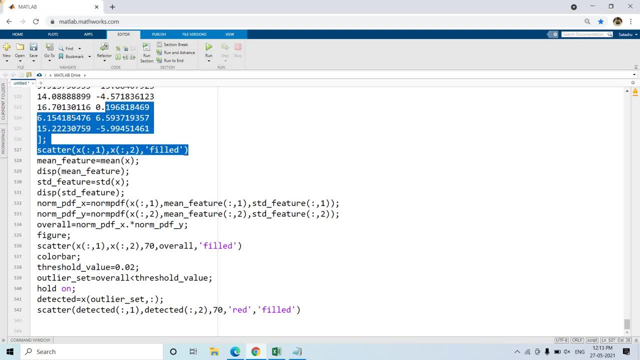 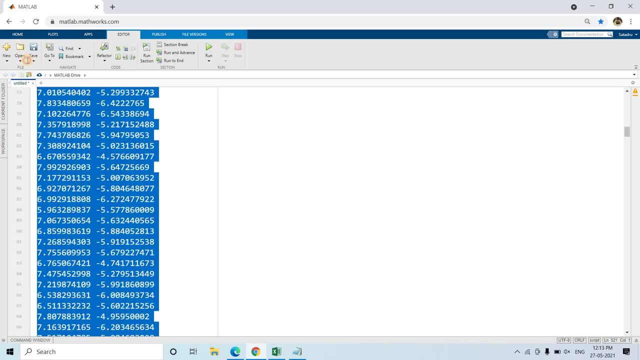 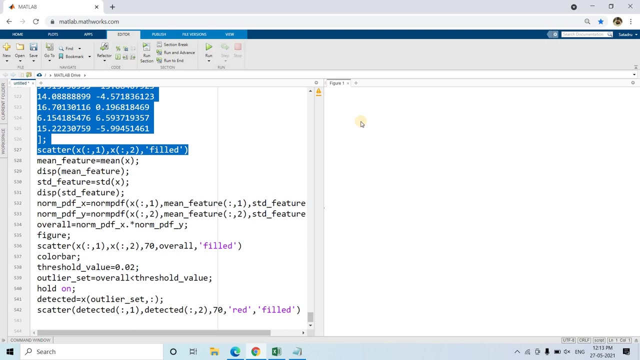 So scatter plot of the data we want to do. let me just run this particular part and show you, so it might take some time. we have to wait. yes, See here in figure 1, this scatter plot we can see. So this is our x2 feature in y-axis. x1 feature in x-axis. 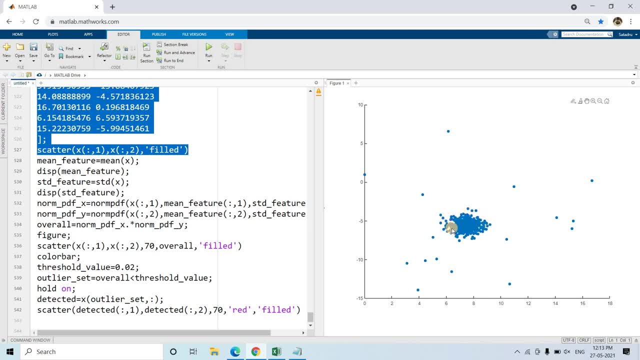 We can see that. So this is our x2 feature in y-axis. x1 feature in x-axis. So this is our x2 feature in y-axis. x1 feature in x-axis. We can clearly understand that most of the data points are concentrated along this part. 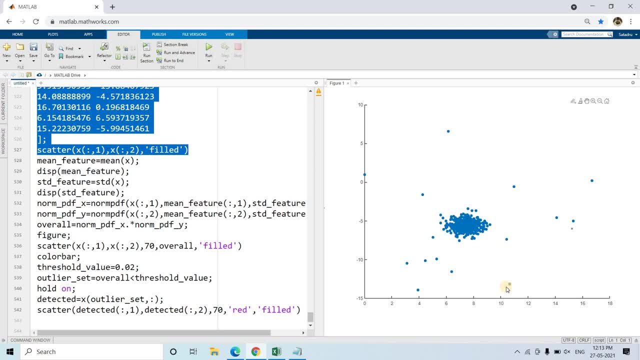 So all these data points, wherever I am moving my mouse pointer, there is a probability that these are outliers. So now let us try to apply the same concept and try to get the visualization. So what is the first step? I have told you that for each input feature, we need to compute the mean and standard deviation. 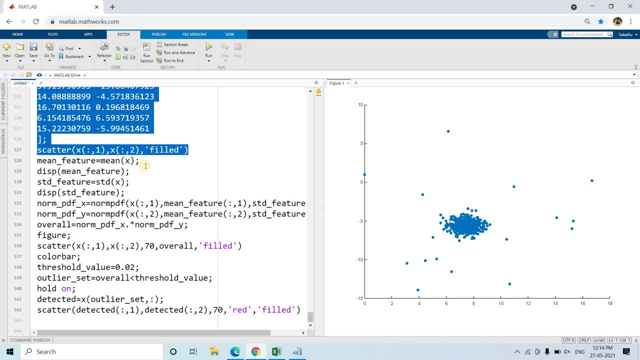 because we need to fit Gaussian distribution for each input feature. we need to compute the standard deviation here, So we need to fit Gaussian distribution for each input feature which is x1,, x2,, x3,, x4,, x5,, x6,, x7,, x8,, x9,, x10,, x11,, x12, x12,, x13,, x14,, x15,, x19,, x20,, x21,, x22,, x23,, x25,, x26,, x28,, x28,. 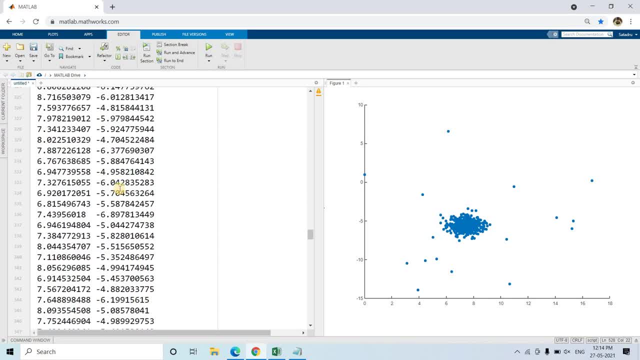 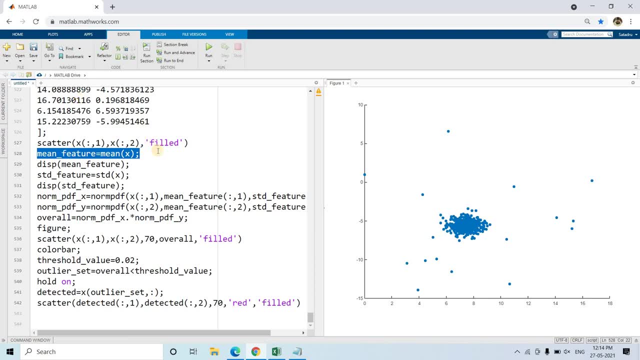 matrix which is storing my input features. okay, and if we use the mean function, it will compute the mean column wise, okay. so for first column and second column there is two inputs. for the two input features you can get the mean if we want, we can display the mean. similarly, we can. 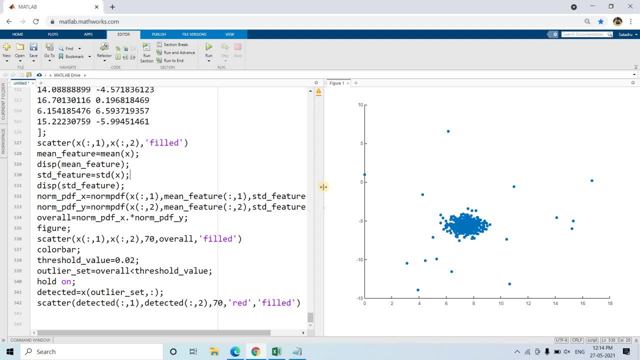 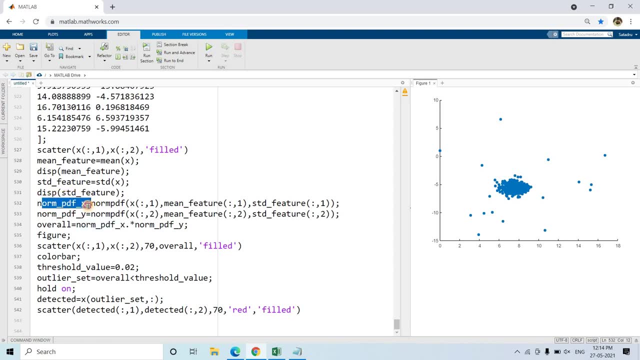 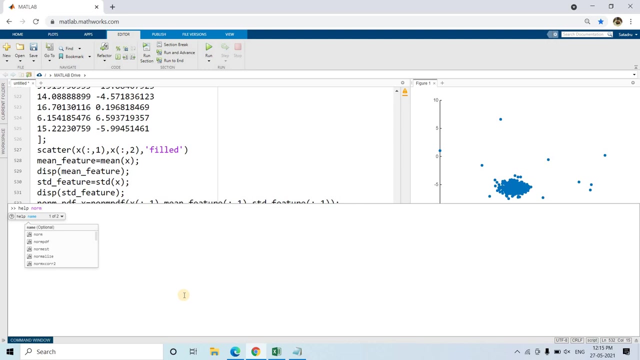 compute the standard deviation here. okay, now we need to fit the gaussian distribution on our first column and second column separately. so norm pdf x: okay, probability distribution function along x axis. norm pdf is the function to fit gaussian distribution. you can simply go in the comment form and write norm pdf- okay, just hit enter and here you can read about this particular function. 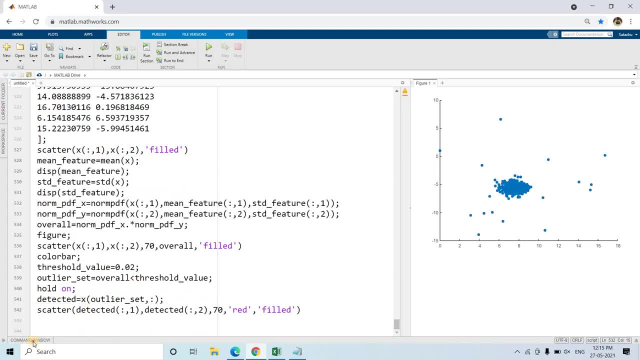 it recent returns. the probability density function of normal distribution- okay, normal distribution with mean mu and standard deviation c, perfect. so here what i have done for x direction, i have given the mean of the x values and standard division of the x values for getting the probability density functions or probability values. for y direction, i am giving the y data points first. 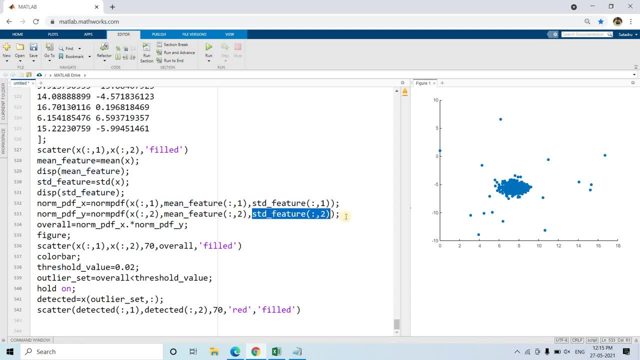 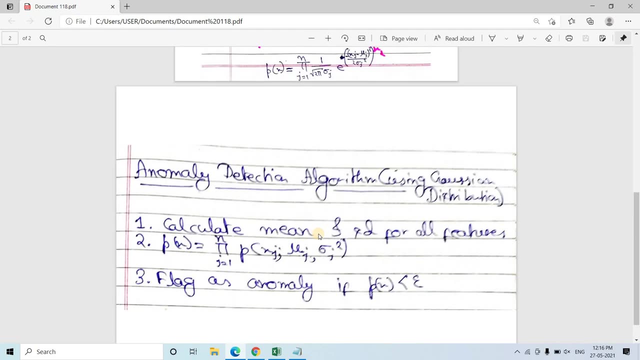 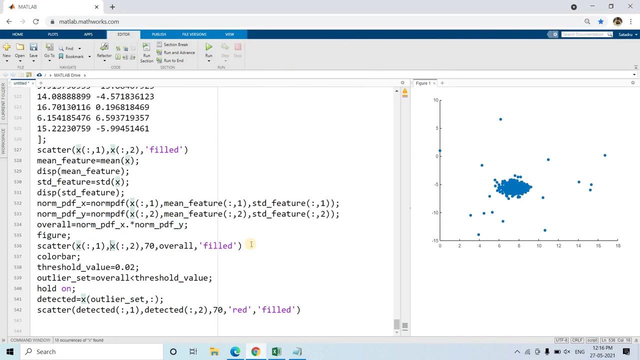 and the mean of y data points and standard division of y data points. okay, so once we get this, individual probabilities of individual dimensions: okay, or individual input features, which is我說, σε, we need to multiply. okay, the same equation which i have just now shown here, that is, to get the overall probability. we need to multiply. okay, right. so once that is done, what we need to do, we can do scatter plot. okay, and here this scatter plot, i am, uh, for colouring purpose, to show the probability values, how those are changing. i am giving here the color as overall- okay, that is overall probability. 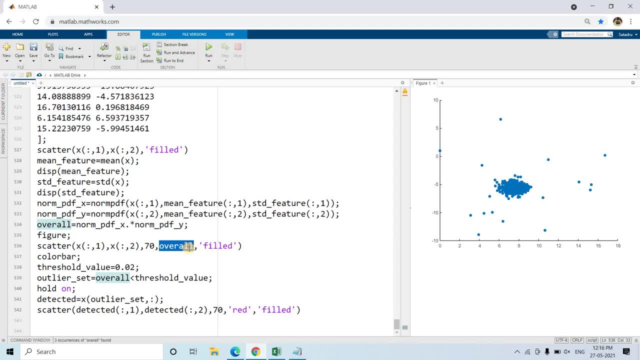 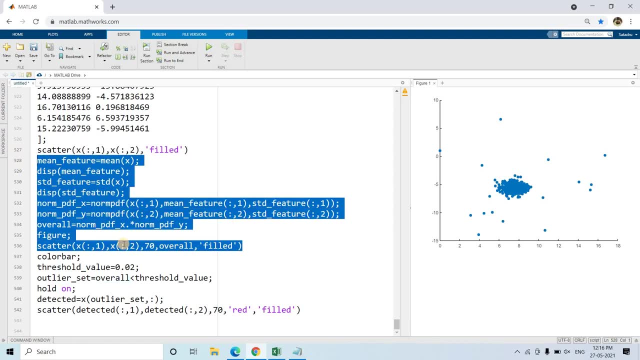 the color. okay, right, the yellow color region will be having higher probability, the blue color region will be having lower probability, like that. okay, let us check. so here we can run this particular part only because after this we ran already. so here just we need to do evaluate selection in. 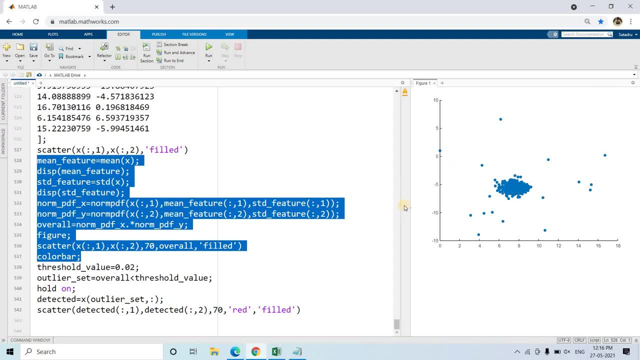 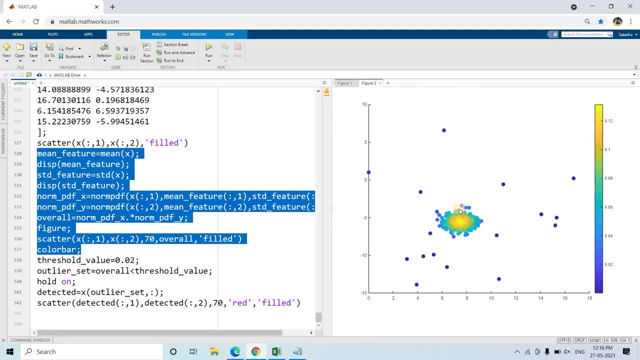 comment window. okay, so in a new figure window we can see the data points, but it will give the color according to the probabilities. higher probabilities will be having yellow color, like see here. so as we just intuitively try to understand using mathematics, here most of the data points centered. 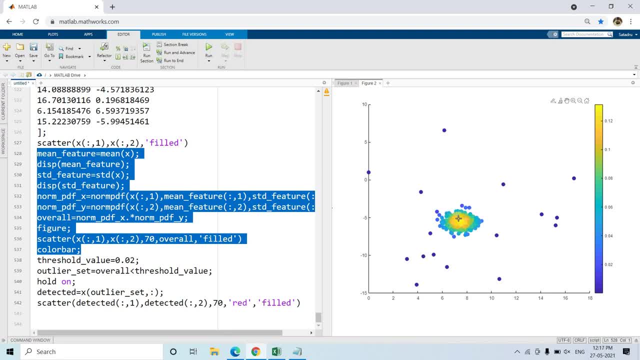 around this. so probability, overall probability after multiplication will be more along these centers. so these are having yellow colors. you can see the color bar. okay, more probabilities: 0.12. close to that is yellow color and as we are moving away, that is anomaly parts or outliers. parts are: 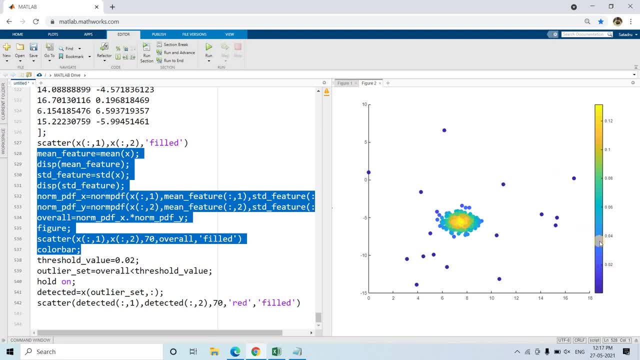 having blue color. see, blue color is having less probability, 0.02, like that. okay, the color bar is clearly showing that. now what we need to do: once we get the overall probability, we need to specify a proper threshold and then we need to detect those anomalies. okay, 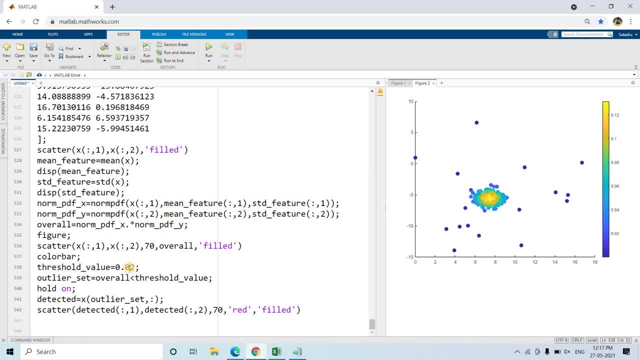 so threshold values equal to 0.02 i am choosing in this particular case. the threshold value has to be chosen very wisely, based on the business use case, okay, and the proper tuning has to be done, otherwise it might happen. improper choosing of threshold value may lead to such scenarios where 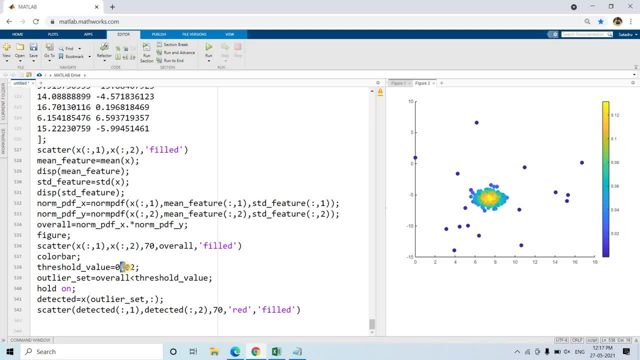 anomalies will be considered as a possibility and the threshold value is going to be 0.02 as normal data point or normal data points into mass. let us analyze, okay, so you need to choose the threshold value very, very properly by trial and error method. you can go ahead or cross. 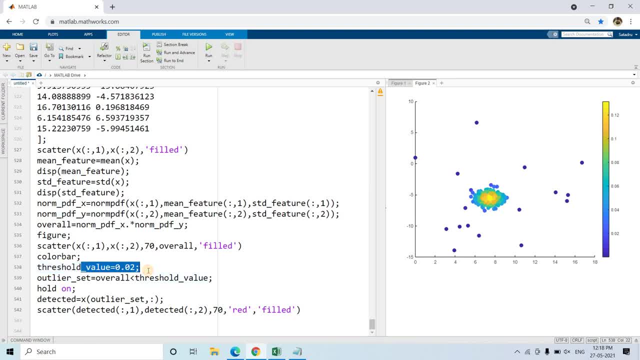 validation. you can use, okay, threshold value equal to 0.02. we are specifying for our this case, outlier set equal to: if the overall probability less than the threshold values and if the overall probability less than threshold values. we are taking those data points and we are plotting. 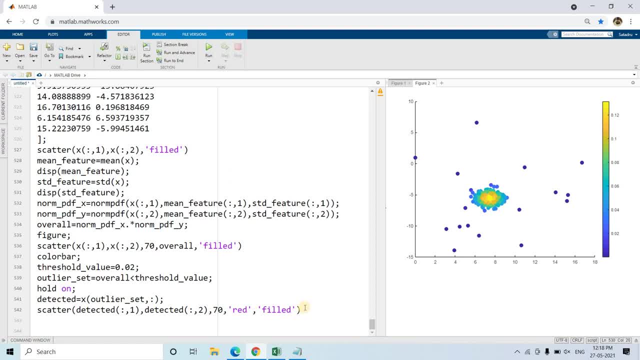 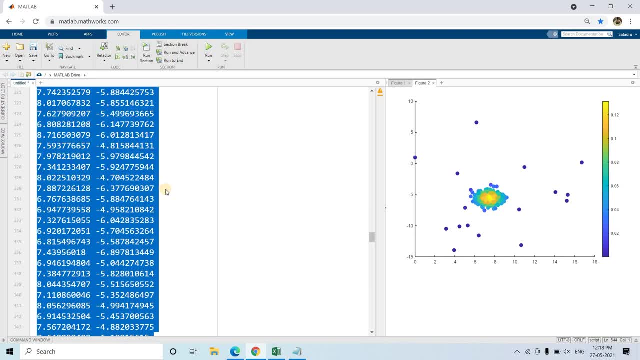 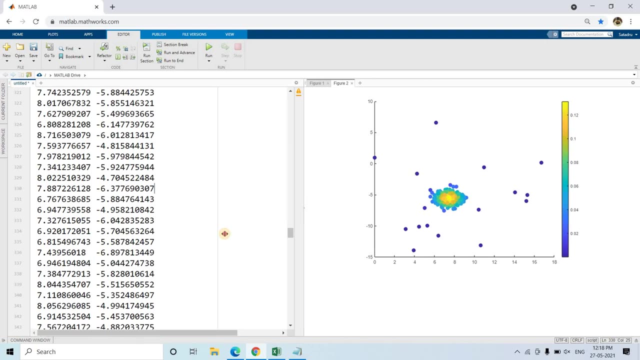 in red color. okay, so now what we can do, we can just uh plan basically the full code notion that let me just do ctrl a and then do failure selection. so eventually what will happen? that all the anomalies will be detected as red color. okay, so here this figure one is our input data points. okay, 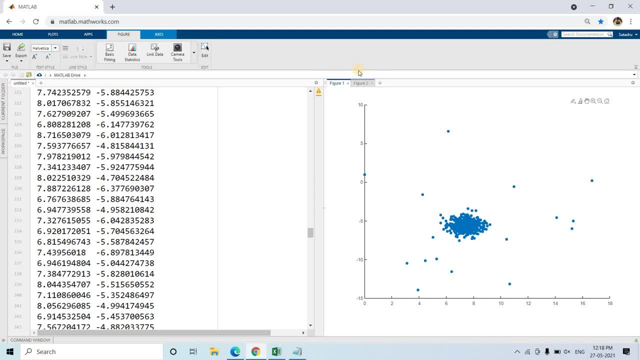 well, we need to detect the anomalies. from the visual inspection we can say these are anomalies, but if you check the figure two here, we can clearly understand that how beautifully the anomalies are detected using multi-dimensional gassian distribution. okay, because this is in two dimensions, we are trying to fit gassian distribution and we are trying to get p of x1. 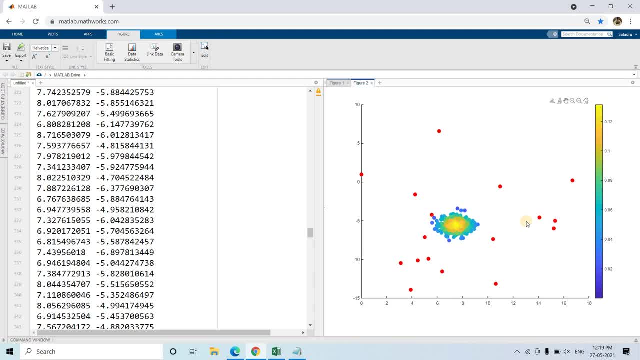 comma x2. okay, in this case that is nothing but p of x1 multiplied by p of x2, because those input features are independent. but, uh, we can understand how beautifully these anomalies are detected. see, all these red data points are anomalies or outliers in two dimensions, and these are basically our original data one. that is normal event. okay, right, and 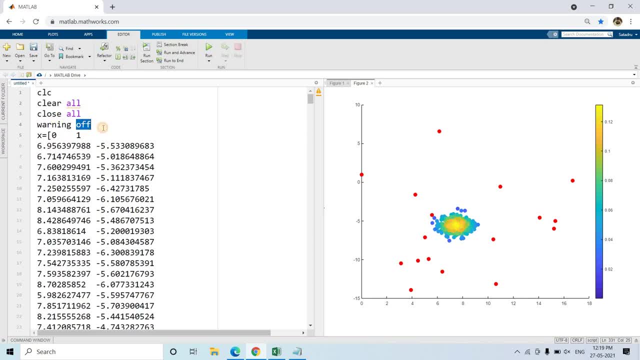 suppose in interview you were asked: what is uh? what type of machine learning is this? there is no doubt this is unsupervised machine learning. you may ask why? simple here, we are not having labels in our data. okay, so in that unlabeled data, our machine learning is trying to detect the data.